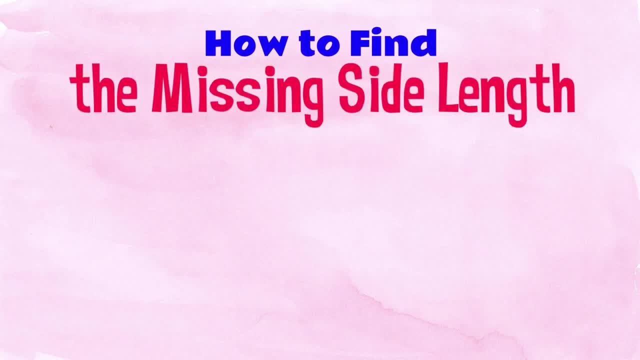 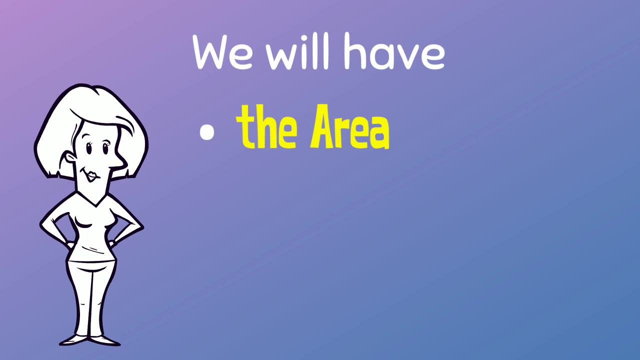 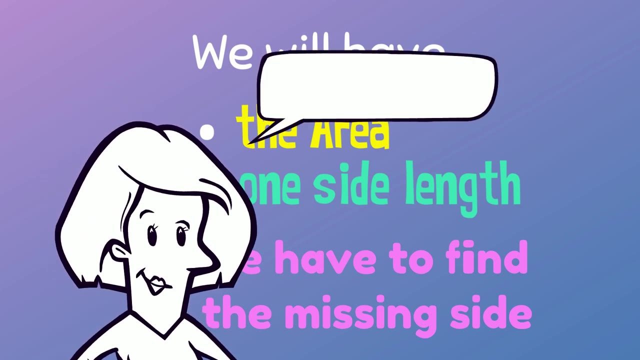 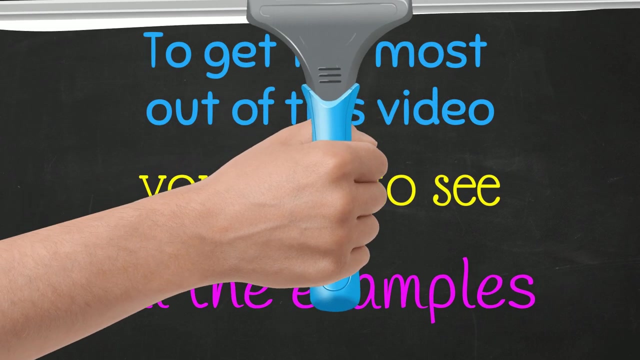 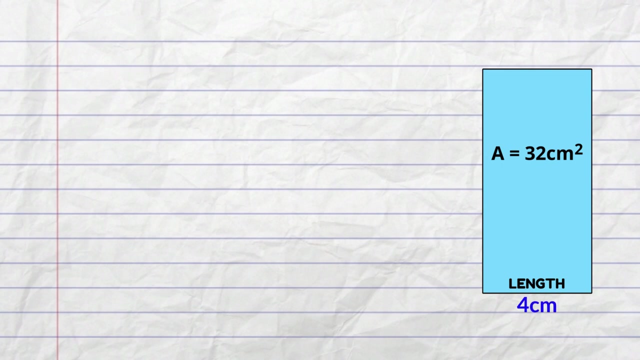 HOW TO FIND THE MISSING SIDE LENGTH OF A RECTANGLE WHEN YOU KNOW THE AREA. As with all my videos, the examples build in complexity, So to get the most out of this one, you need to see all the examples. The length is 4cm. 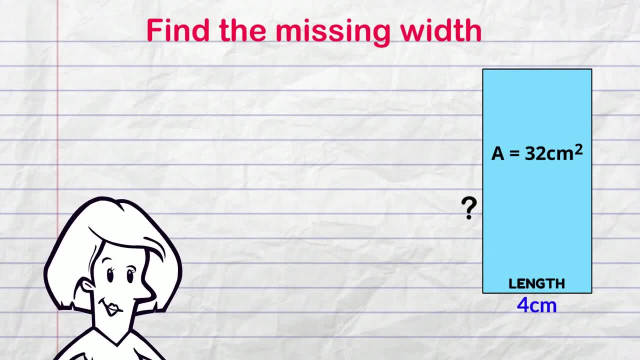 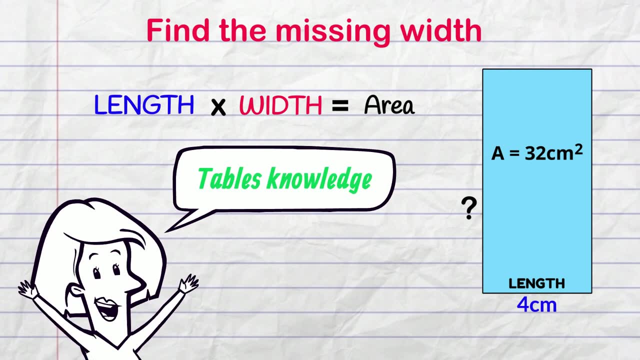 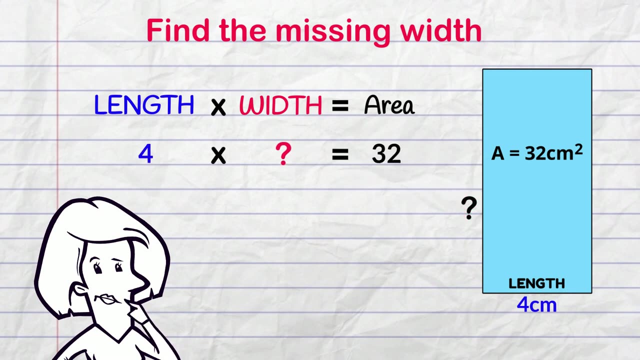 We have to find the width We know. we multiply length and width to find the area. We can solve this problem using our TABLES knowledge. The question I ask myself is: 8cm is the missing side length? Do you see how, knowing your multiplication tables? 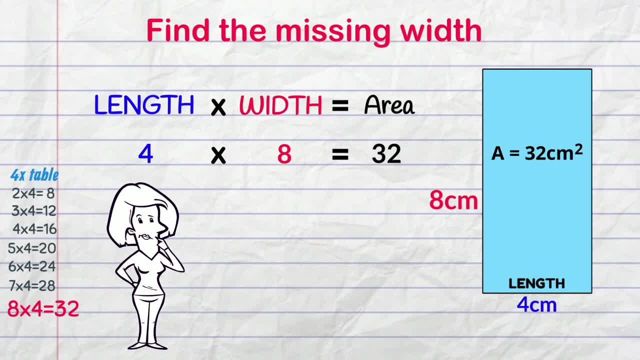 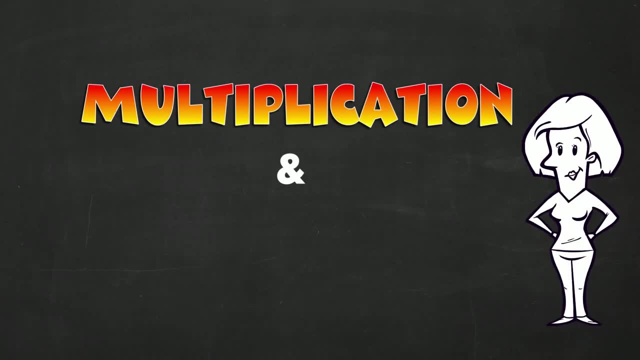 can help you get straight to the answer. If you haven't learned your tables yet, it's time You need this. As you know, multiplication and division are inverse operations. They are opposites. So you can use multiplication or division to solve this kind of problem. 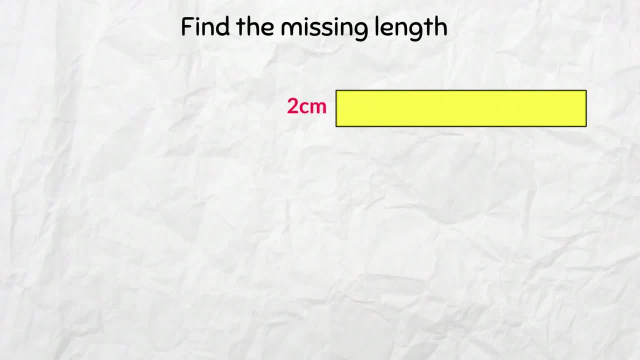 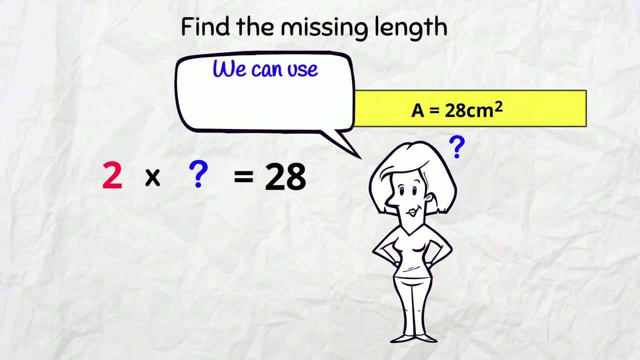 In THIS rectangle we have a side measuring 2cm and an area of 28cm2.. So 2 times some number is 28.. 28 is NOT in our 2x table knowledge. We can use DIVISION to solve it. 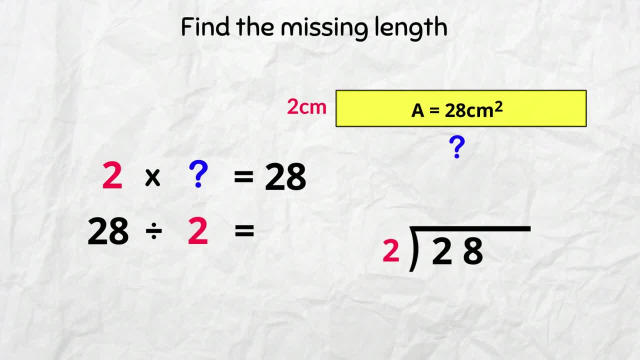 28 divided by 2 is the length of this side. How many 2's in 2?? 1, And how many 2's in 2?? How many 2's in 8? 4? 2's are 8.. 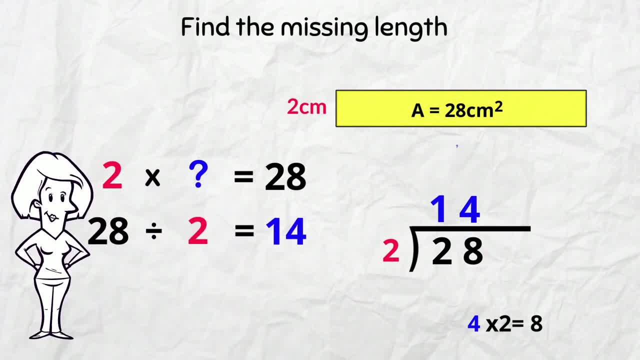 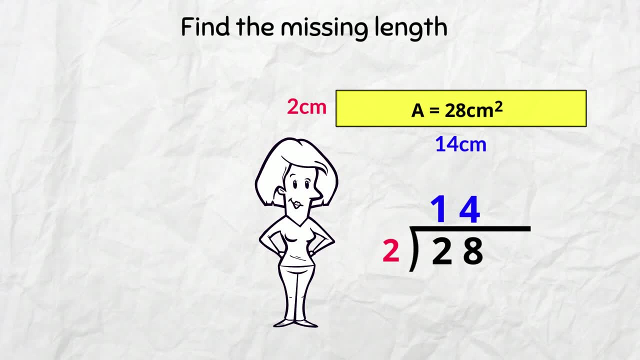 14 then. So this side is 14cm in length. That wasn't too tricky. Yes, the area value was outside our 2x table knowledge, but it worked out perfectly with NO remainder. But you've guessed it, It won't ALWAYS work out perfectly.